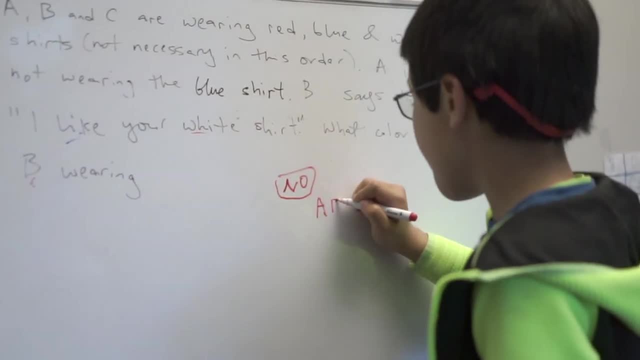 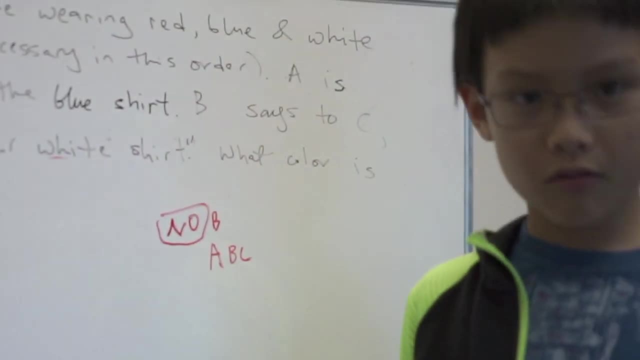 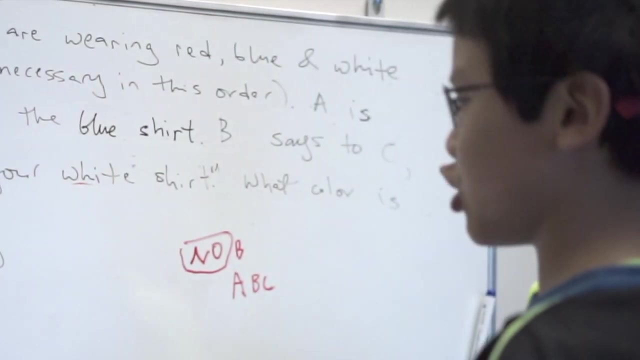 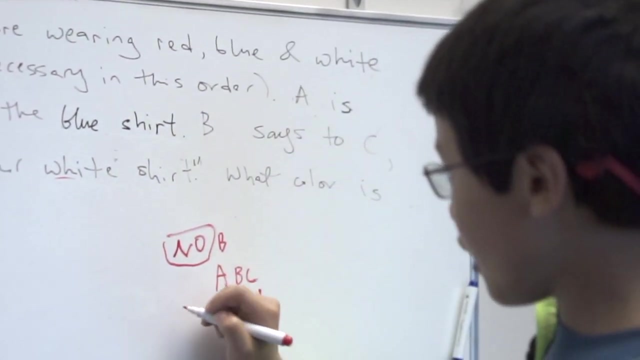 let's write the letters A, B and C, So not wearing blue. So put B on top, which means that A is not wearing blue. B says to C: I like your white shirt. So it means C is not wearing blue, C is white, meaning a white shirt. So we put a W here and write yes. So 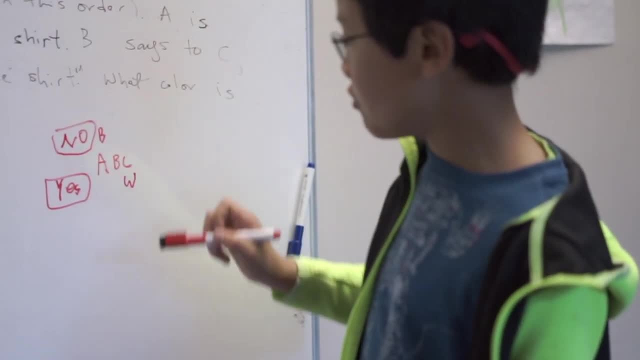 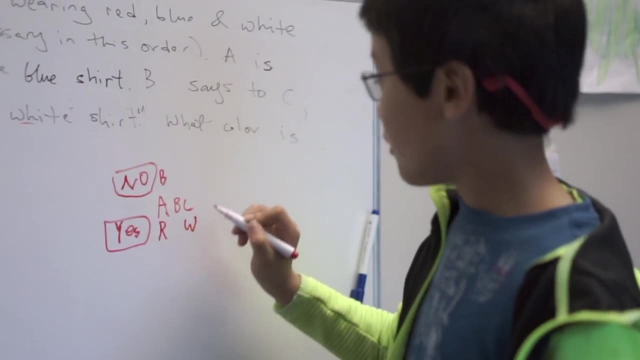 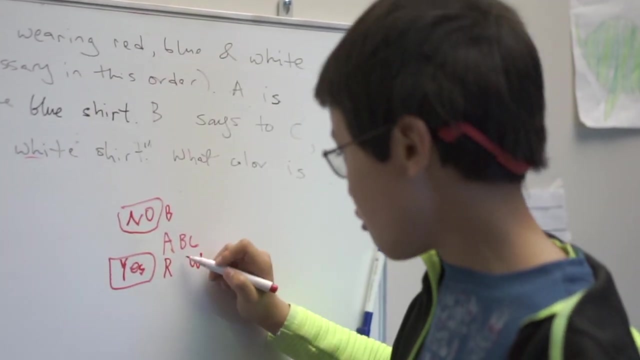 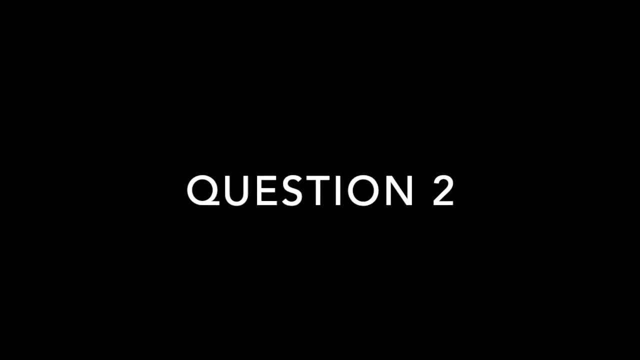 I'm solving for A now. So it cannot be blue or it cannot be white, So therefore it must be red. So let's put red here. So since red and white are taken, we know it got to be blue. So B is wearing blue, and blue is today's answer. 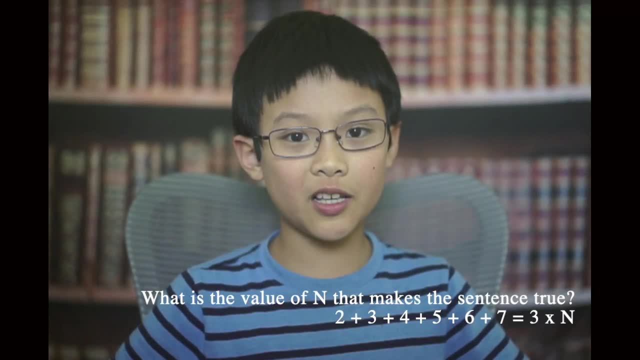 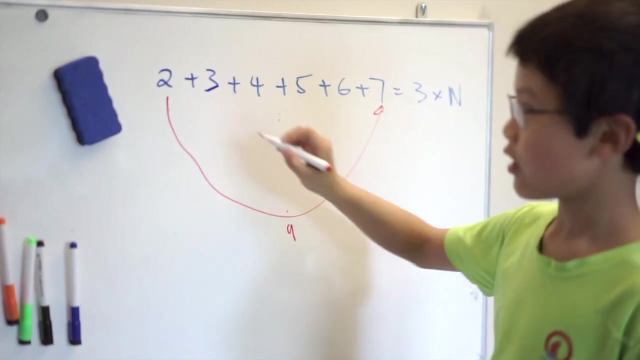 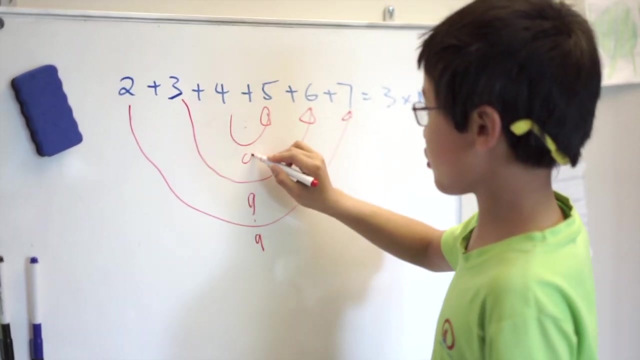 What is the value of n? that makes the following sentence true: Two plus three plus four plus five plus six plus seven equals three times n. I noticed that two and seven equals nine, and three and six Also equals nine. And then I do four and five, which equals nine, Since there are three pairs. 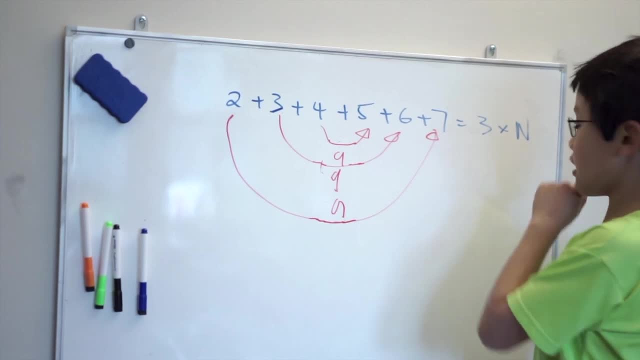 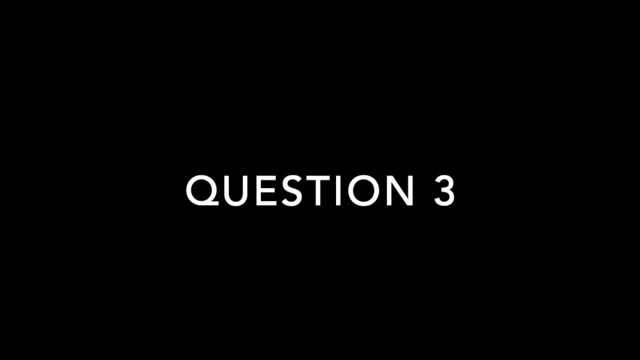 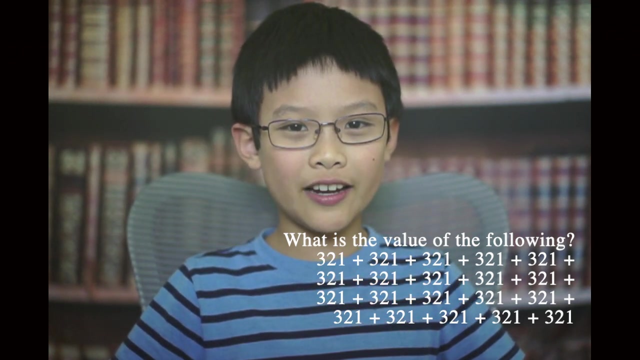 of nine and there are also three pairs of n, so it means that n equals to nine. What is the value of the following: Three two one plus three two one and so on? For this problem, we need to find out how many three- two ones there are. 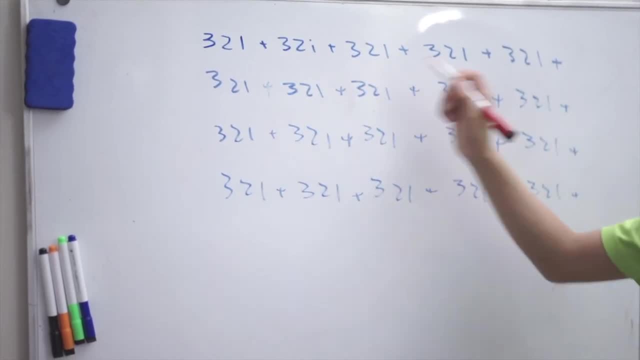 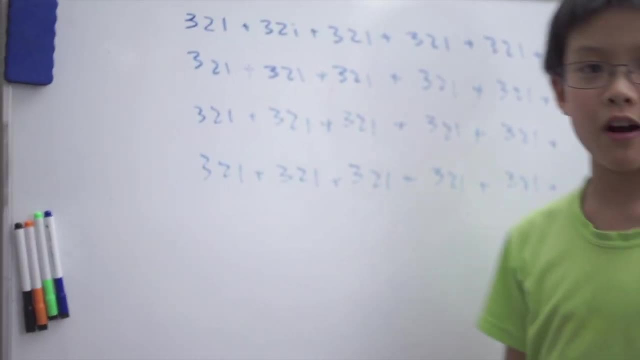 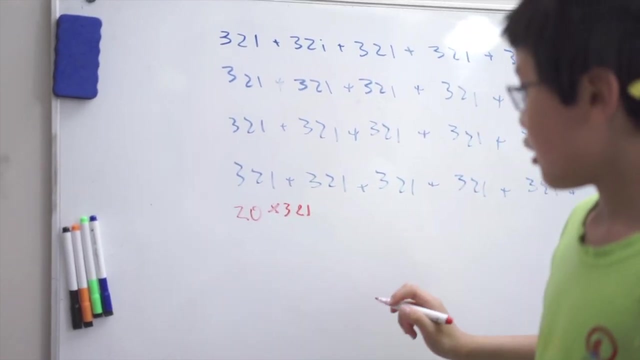 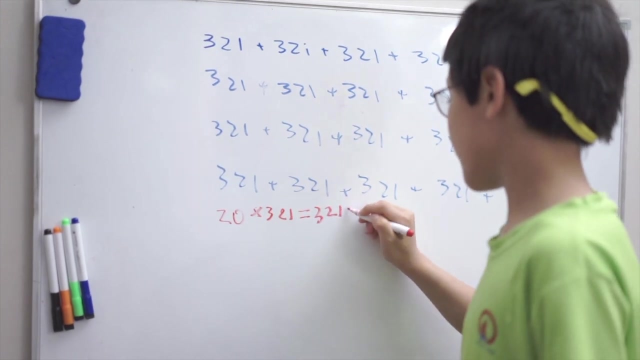 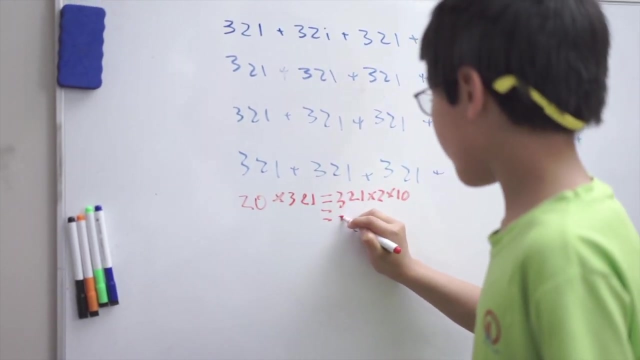 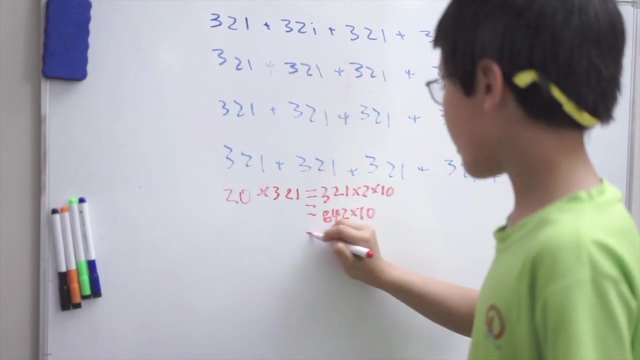 Since there are four rows and five columns, we have to do four times five. So there are twenty three, two ones Twenty times three, two, one. To do that, this equals to three, two one times two times ten, which equals to 6,. 4, 2, times 10 equals to 6,420..